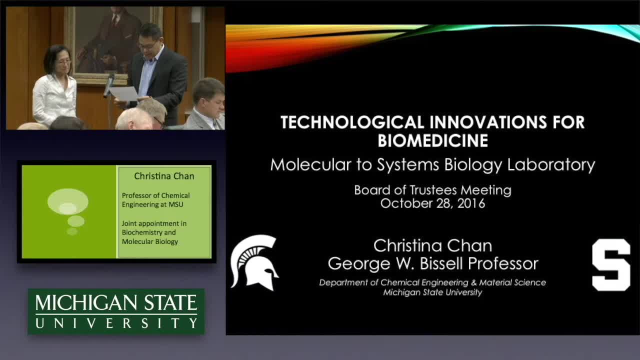 election to fellow of the American Institute of Medical and Biological Engineering, AIMBE, in 2012.. She has mentored over 60 undergraduates in research projects in her lab over the last 14 years at MSU, about half of whom were women. These undergraduates have gone on to graduate. 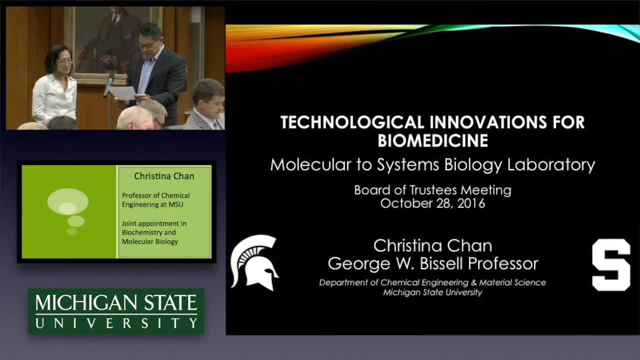 and medical school and also into industrial positions in chemical engineering, pharmaceutical and biotech companies. Welcome, Christine. Good morning and thank you for the introduction. It's my pleasure to share with you some of the biomedical research that's ongoing in our laboratory. So the research. 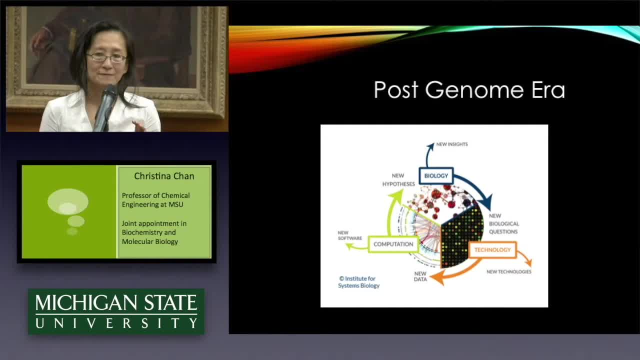 in our lab actually encompasses three focus. The three focuses are computation, biology and technology. So in our lab we develop, as well as use, computational models to analyze the data and to provide new insights into the rules of biology, which then requires. 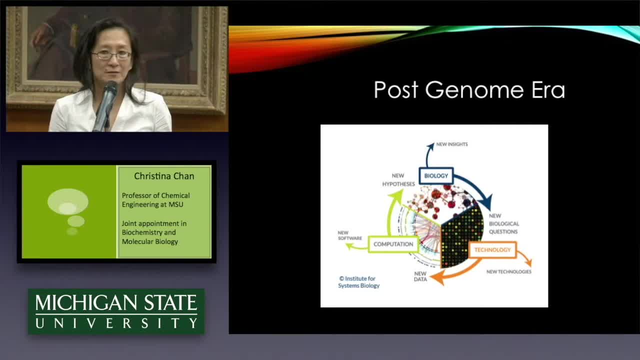 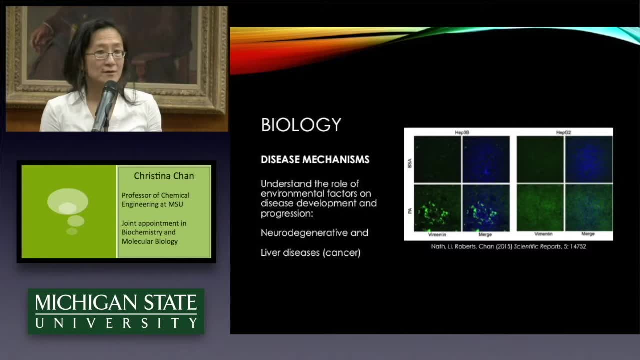 if we want to further investigate these new insights, that we develop new technologies. So one of the focus in our laboratory is to try and understand the role of environmental factors in the development and progression of diseases such as Alzheimer's and liver cancer. We know that, or it's been suggested in. 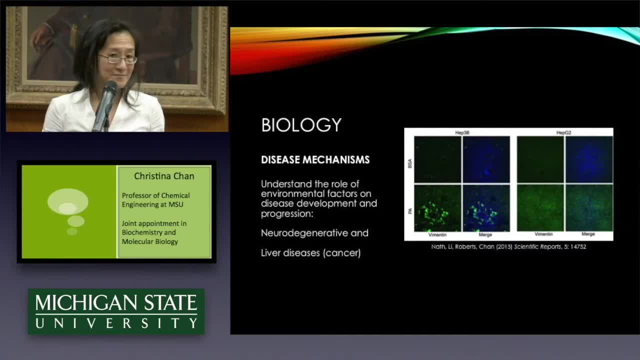 epidemiological studies that obesity is highly associated or linked with a liver tumor genesis and increased mortality, as well as a number of other diseases. However, we actually analyzed liver samples from cancer patients and found that BMI is not associated or is not a very good predictor of the progression of liver cancer. 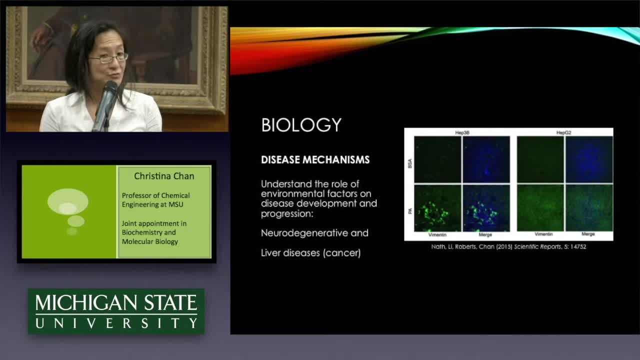 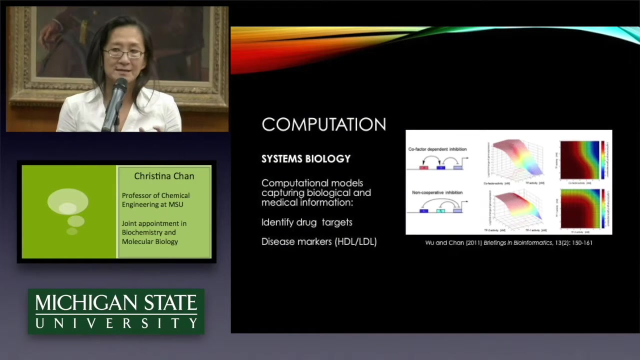 Instead, what we did identify was a scavenger receptor protein that is involved in taking up fatty acid. that is a good predictor and, furthermore, contributes to the progression of liver cancer, And so that highlights the importance of gene-environment interactions in the progression of diseases. And so to understand the role of these environmental 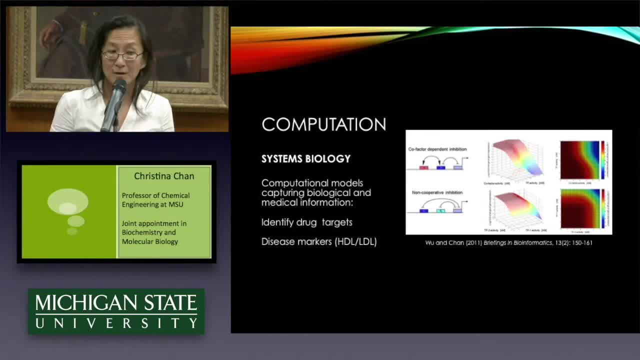 factors. our group also developed computations. So the idea there is to ask the question: how do the network of pathways change to give you the particular phenotype that you see, in order to identify, in our case, novel pathways that could be potential biomarkers as well as drug targets? 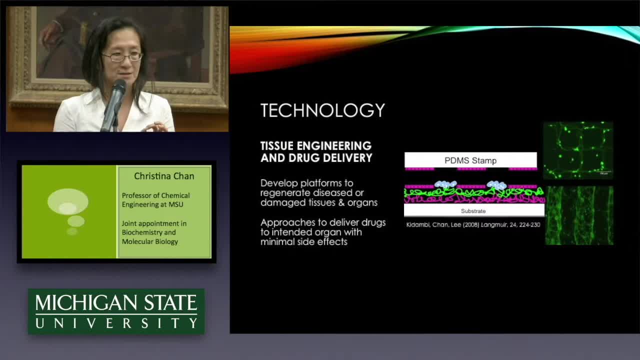 And so to really determine whether these pathways have disease-modifying effects typically requires one to perform animal or cell culture studies. Now, one of the issues with cell culture studies, or rather with in vivo animal studies, is the fact that you have a lot of complex interactions that go on that make it very difficult to 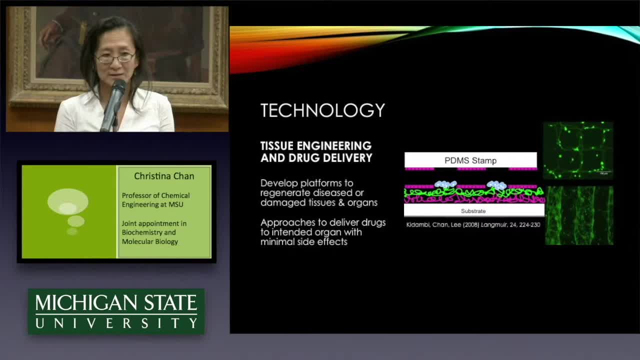 assess the exact contributions of the pathway that you're trying to study. However, when you look at cell culture study, the limitation is, or the challenge is, that oftentimes the response you get in the cell culture study doesn't necessarily correlate well with the cell culture study, And so that's one of the things that we're trying to do. 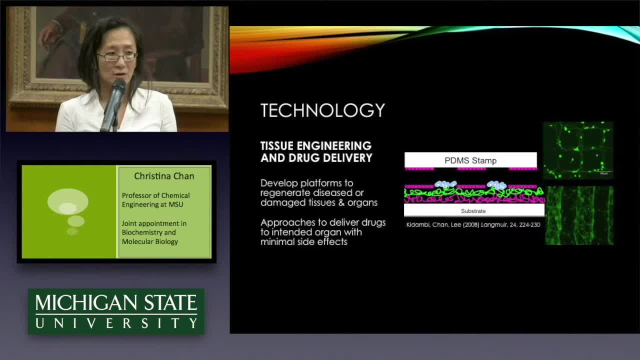 And that's what we're trying to do with in vivo response. So one of the things that our lab is working on developing are these biomimetic systems that can take into account cell-cell and cell-surface interactions, so that they can better recapitulate. 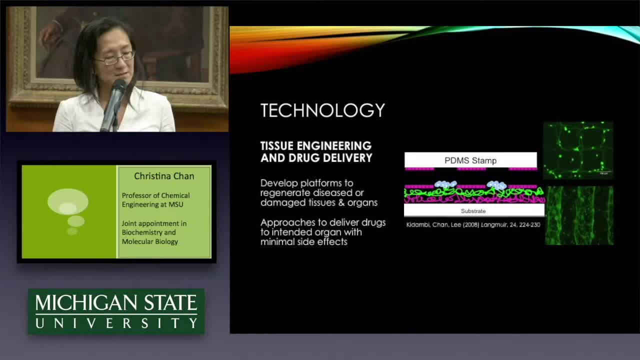 the microenvironment, so that now, when we test these pathways, it would better be able to correlate with the responses that you see in vivo. So in the next three slides, what I'd like to do is briefly cover some of the things or some of the projects that were performed or are ongoing in our lab. 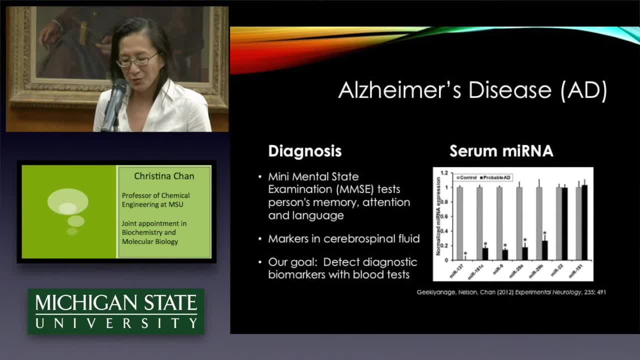 So one has to do with the diagnosis of Alzheimer's. So currently the way to conclusively determine whether a patient has Alzheimer's disease is by analyzing the biomarkers in the brains of post-mortem AD brains, which is a little difficult to do with live patients. 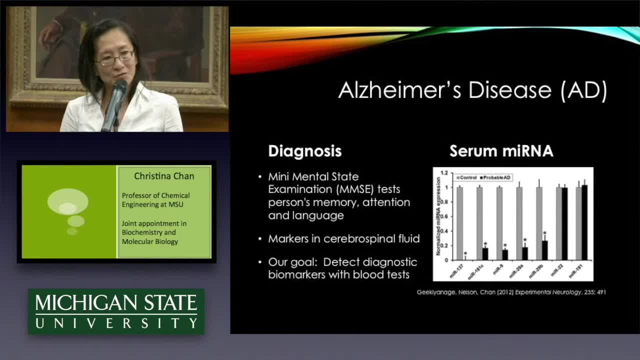 And so now the typical approach that people use is a more qualitative approach. So we're going to talk a little bit more about the qualitative approach of cognitive tests, which essentially is one, for example, the mini mental state exam, which is a questionnaire. 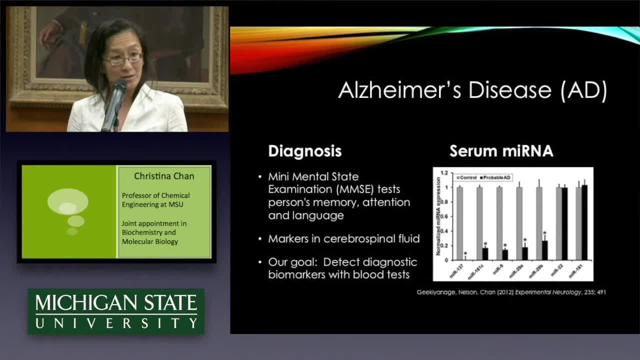 that is used to assess a patient's memory, attitude and language skills, for example, And so the challenge there is that once you take those exam, it can tell you that the patient may have dementia, but it doesn't necessarily distinguish whether the person 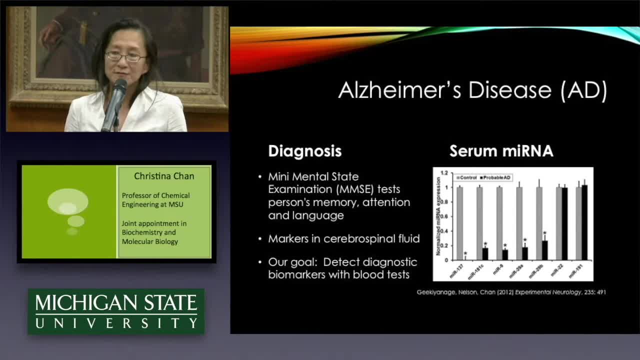 has AD or some other form of dementia. So, alternatively, there is a study that's going to do another approach, where you can take cerebral spinal fluid from the patient and analyze the biomarkers, which is more conclusive in determining whether a patient has AD. 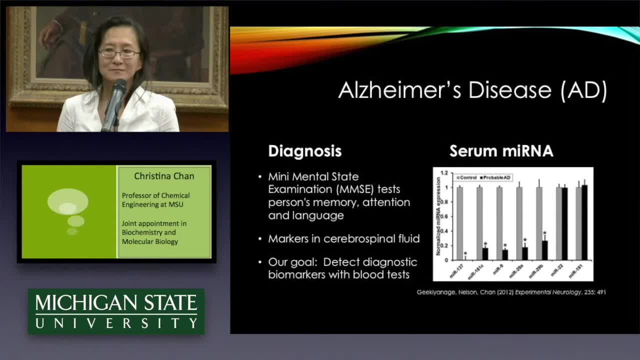 However, it is a highly invasive procedure, And so what we've done is we've taken samples- post-mortem samples- from AD patients and have found that there are these biomarkers, or microRNAs, that are involved in regulating a lipid pathway that is highly reduced in. 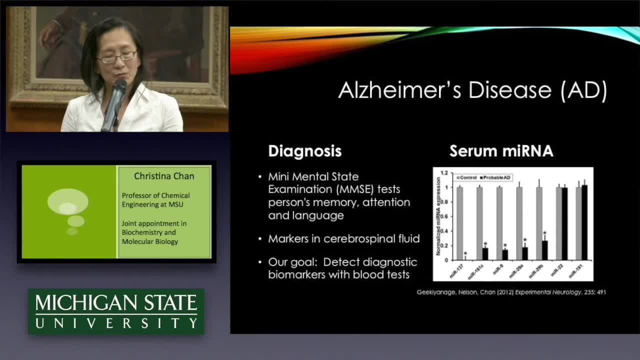 the brains of AD patients And, surprisingly, what we found was that these same biomarkers are also significantly reduced in the blood serum of patients, of AD patients. So that suggests that perhaps this could be a potential viable, non-invasive way to diagnose whether. 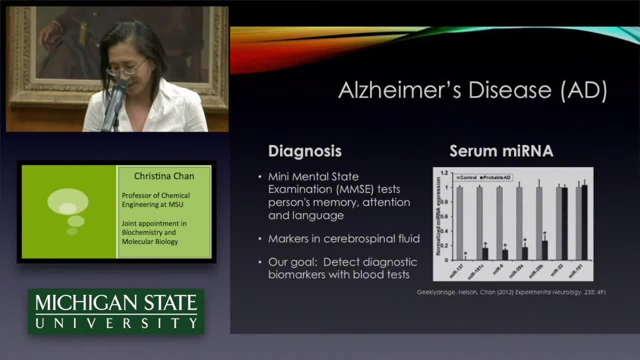 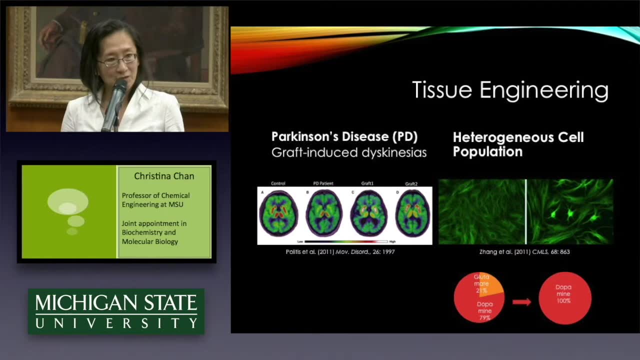 a person has AD. So now shifting gears a little bit. another project that we're actually performing now that we're very excited about It involves CRISPR technology, or gene editing, if you will, applied to Parkinson's disease, And so case studies have shown that when you take fetal grafts and transplant them into 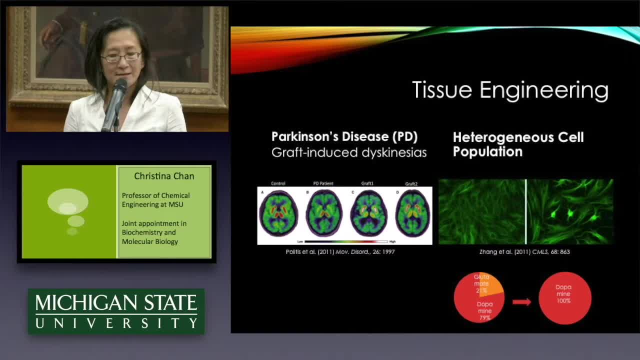 the brains of Parkinson's disease patients that a large percentage of these patients develop a certain side effect, which is these involuntary muscle movements. So it turns out, when they went back to look, they realized that the reason that they were able to do this was because they were able to do this with the brain cells. And the reason for 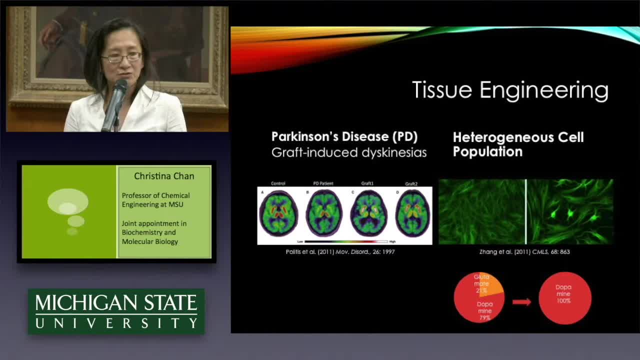 that is, in the transplanted region. the brain cells are not necessarily just producing dopamine, which is what's missing in PD patients, but also other neurotransmitters such as serotonin, And so what we're trying to do is to use CRISPR technology or gene editing to edit. 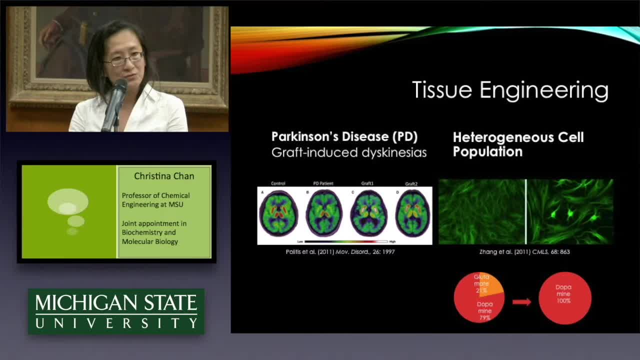 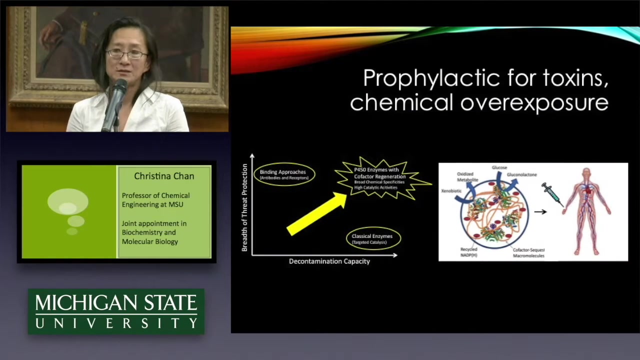 out in neural stem cells their ability to produce some of these other off-target, if you will, neurotransmitters. So the idea is that then, if you transplant these edited stem cells into the brain of PD patients, they will then produce just dopamine. Okay, And the last project that I want to briefly touch upon is a project that came. 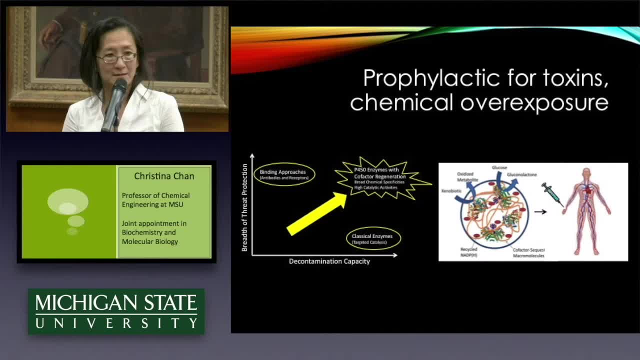 about last year, while I was on sabbatical at Columbia University. And so here the idea is to develop an enzymatic particle for detoxification. And so the idea is to develop an enzymatic particle for detoxification. And so the idea is that if someone were to inadvertently or purposefully be exposed to high level of 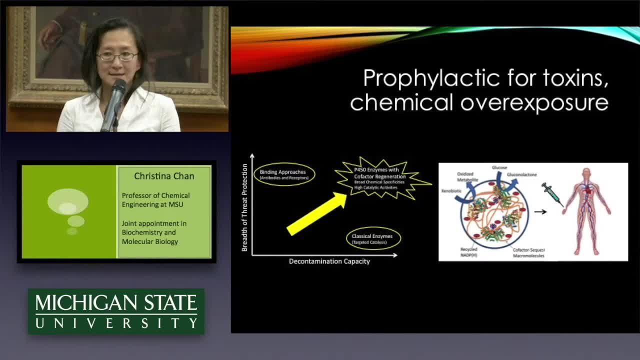 toxins such as, let's say, dioxin, insecticides or even drugs or any molecules that can be used as a threat agent. the idea is, can we develop these enzymatic particles that can be injected into the patient to detoxify these high levels of toxin? 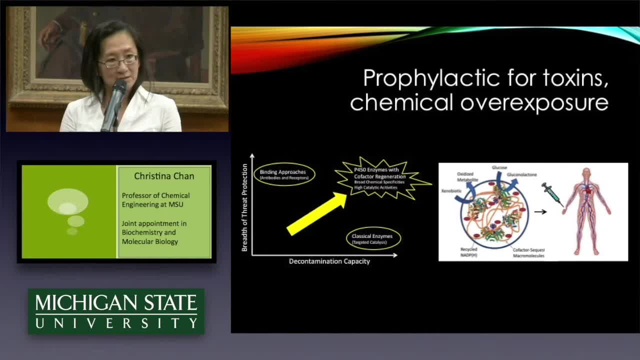 Now, current approaches that are used to address these threats include, for example, the use of an enzymatic particle to detoxify these high levels of toxins, such as, let's say, dioxin, insecticides or any molecules that can be used as a threat agent, or either what they. 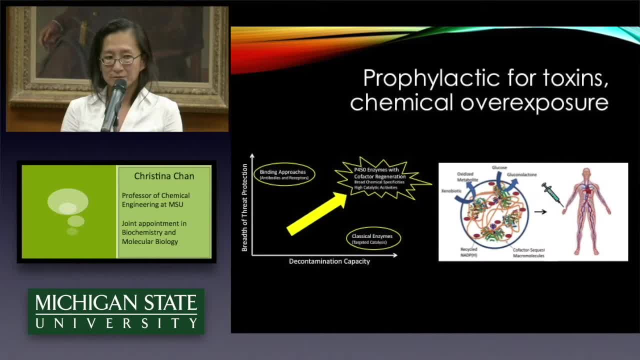 call stoichiometric or catalytic scavengers. So with the stoichiometric scavengers they can detoxify a wide range of nerve gas agents, for example nerve agents. The limitation is that when it binds one of these molecules it becomes deactivated. So the decontamination. 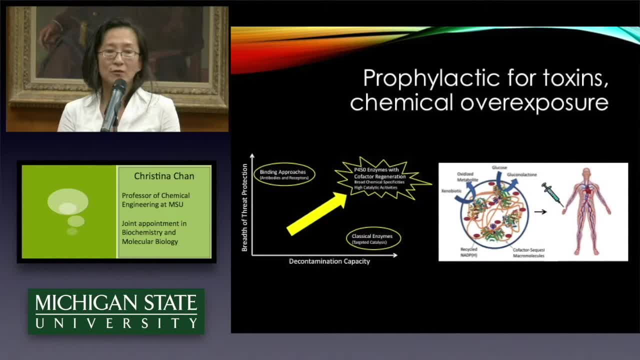 capacity is somewhat limited. So, alternatively, there are these catalytic scavengers that have multiple functional sites that combine many more of these molecules. But the limitation that these catalytic scavengers have is that they can only detoxify a very narrow range of compounds, And so the approach that we're taking is to capitalize upon a particular 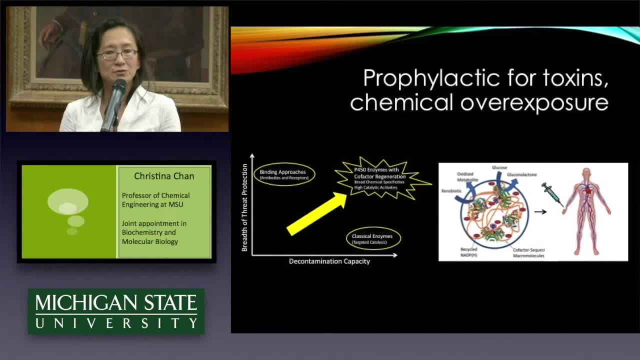 enzyme that's in the liver that is normally able to metabolize and detoxify a whole range of chemicals, And so that, in addition to the breadth of chemicals that they can detoxify, one of the challenges that we're addressing to make this a viable solution is to be able to regenerate the cofactor that is required to maintain.